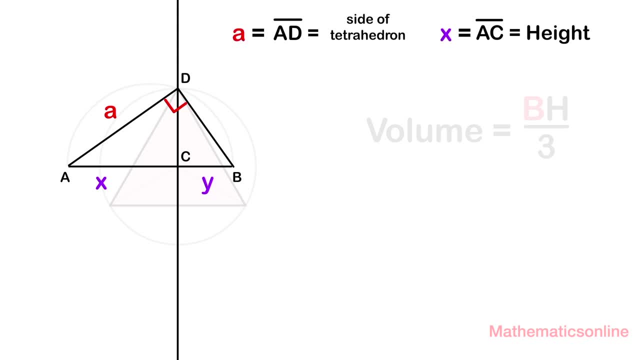 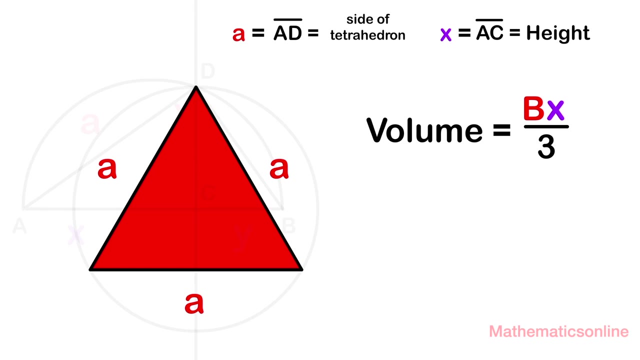 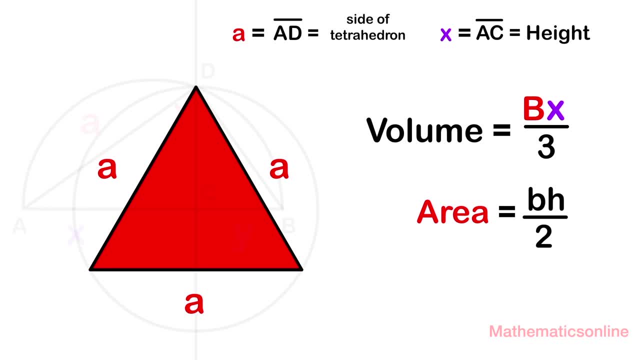 So the base is A and notice that the height divides the base in half, and so we have A divided by two. Notice that we have created a right triangle, and by the Pythagorean theorem, H squared plus A divided by 2 squared is equal to A squared. 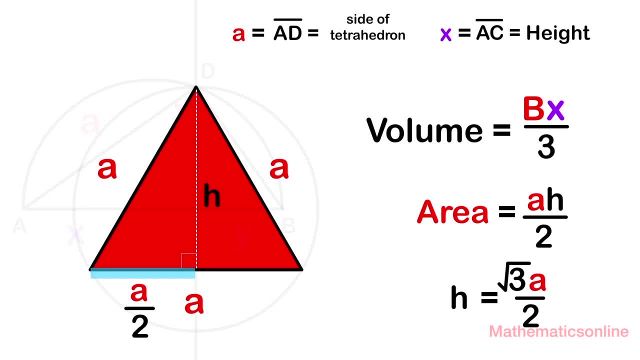 If we solve for H, we get the square root of 3 times A divided by 2, and we'll go ahead and And substitute h above, so the area is the square root of 3 a squared divided by 4.. And finally, let's substitute this into the volume formula. 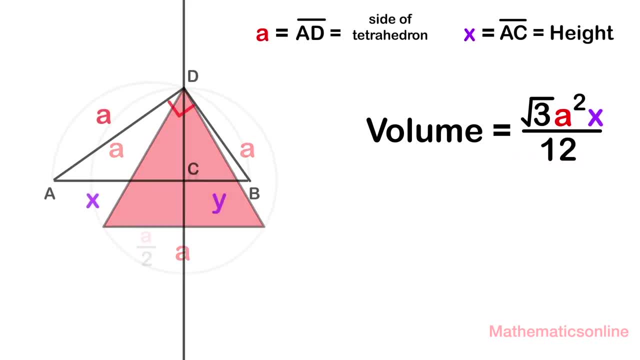 And so we have. the volume is equal to the square root of 3 a squared times x divided by 12.. So we're not done just yet. What we want to do is we want to rewrite the formula in terms of a, So we need to rewrite x. 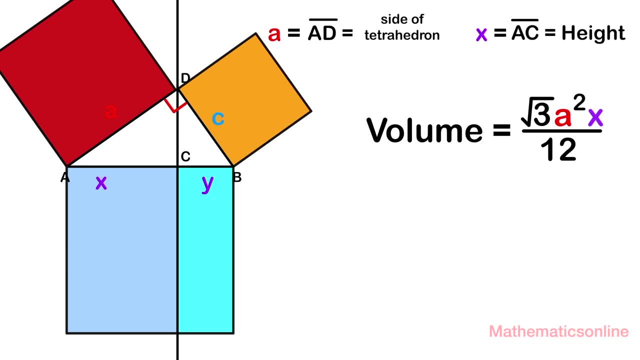 So triangle ABD is a right triangle And from Euclid's proof of the Pythagorean theorem we know that the square on the hypotenuse is equal to the squares on the legs of the right triangle. So line CD cuts the larger square into two parts, and this is how we represent it algebraically. 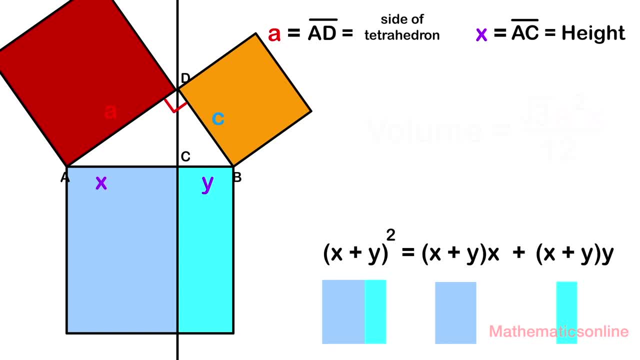 Now, at the very beginning of the construction, we created line AC so that it is twice the length of CB. So this is represented as: x equals 2y. Okay, Let's go ahead and multiply both sides by x plus y. And again, from Euclid's proof, the area of the rectangles are equal to the areas of the.